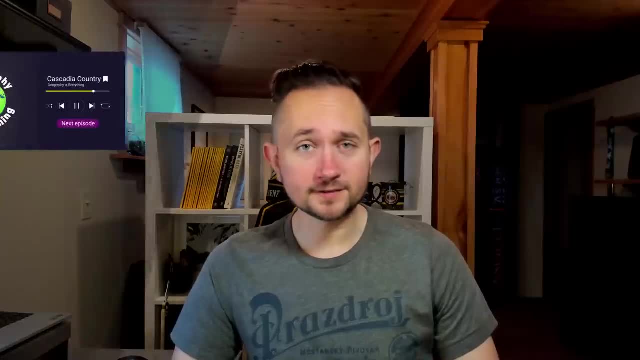 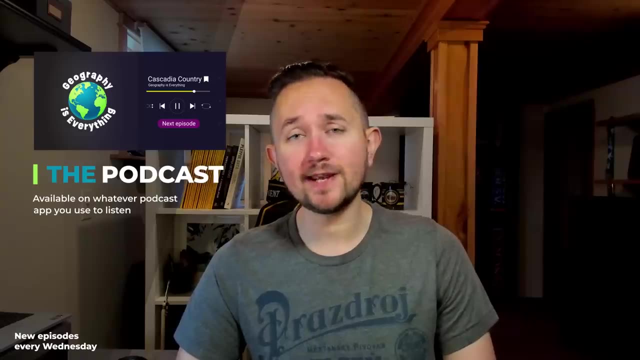 And we're going to explore how that happened in today's video. But, of course, if you're a fan of geography, be sure to check out my podcast, Geography is Everything. New episodes premiere every Wednesday and you can listen Right here on YouTube Substack, where there is exclusive content, or whatever app you use to. 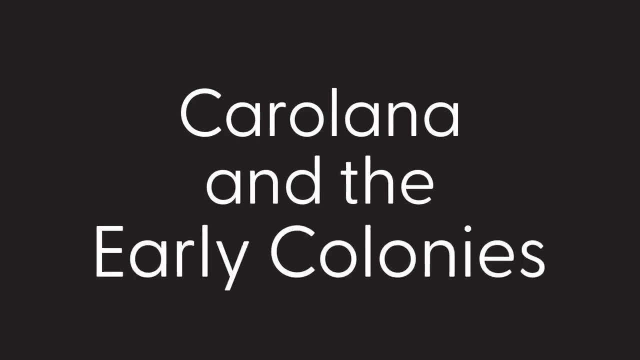 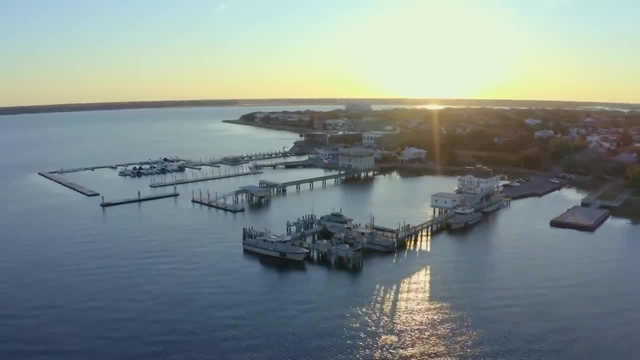 listen to podcasts. The history of the North Carolina and South Carolina split is rooted in the history of how colonies even came to be colonies in the first place, So it's worthwhile to revisit the way in which England handed out charters and mandates for the establishment of 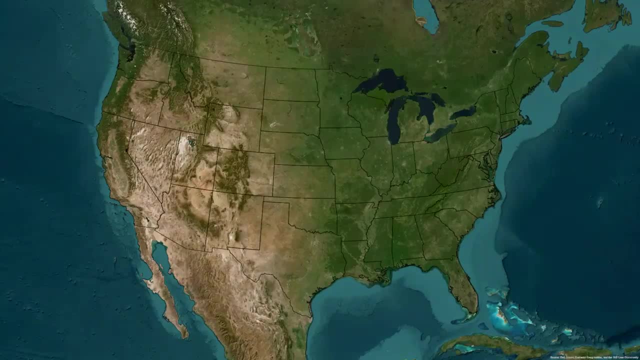 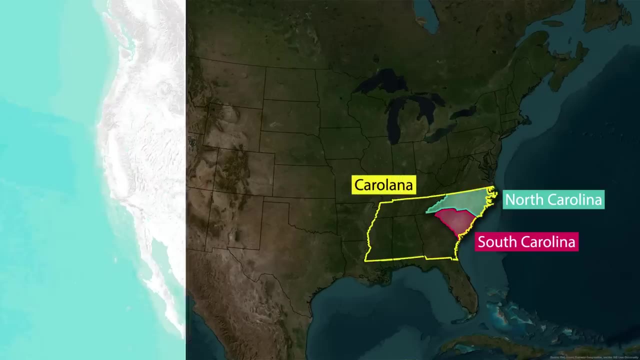 territory within North America. But make no mistake here: North Carolina and South Carolina started out their existence as a single territory, And so we're going to explore how that happened. The story called Carolina. Back in the 1500s, the English monarchy was realizing that it was. 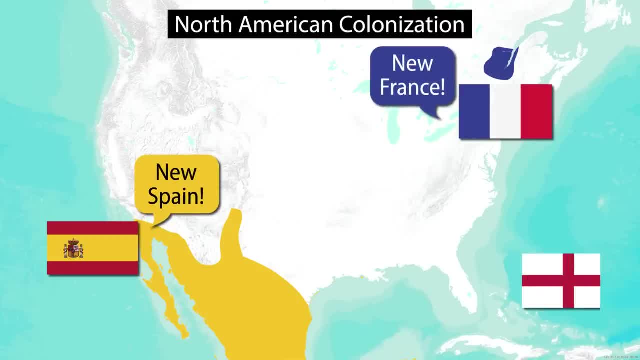 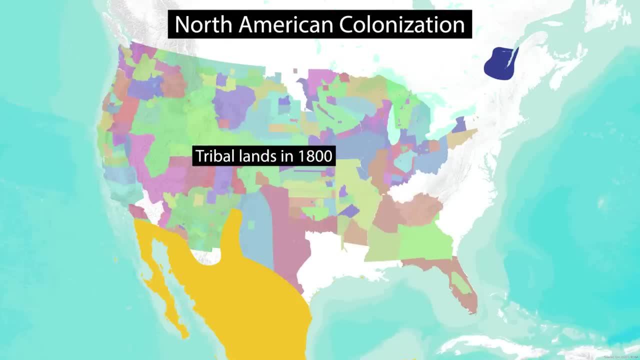 falling behind in the exploration and expansion of its empire in the new world. Of course the Americas weren't new and had actually been inhabited by thousands of different peoples for thousands of years, But that's a whole other story. But England quickly realized that if it was 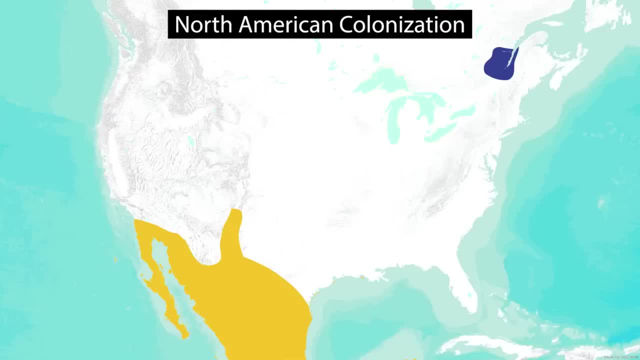 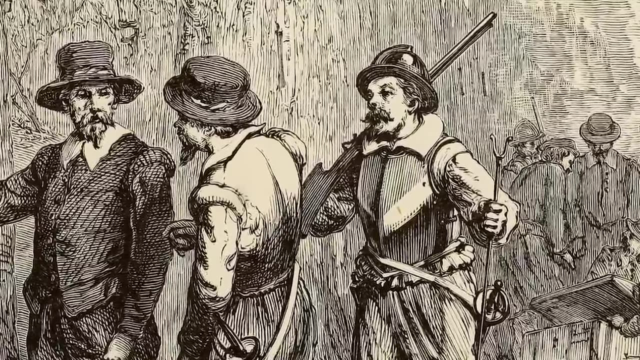 going to compete with the likes of Spain, it was going to need to start establishing its own colonies in North America, And so it began issuing charters to various groups of people who wanted to establish settlements. The first English colony was established at Roanoke, which was founded in 1585.. Unfortunately for 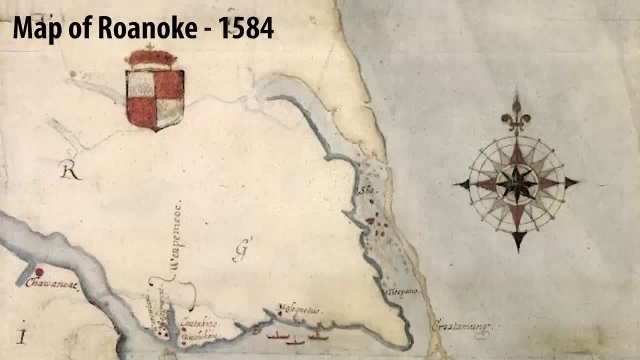 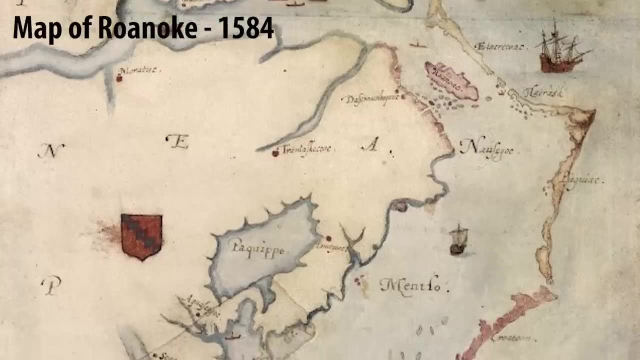 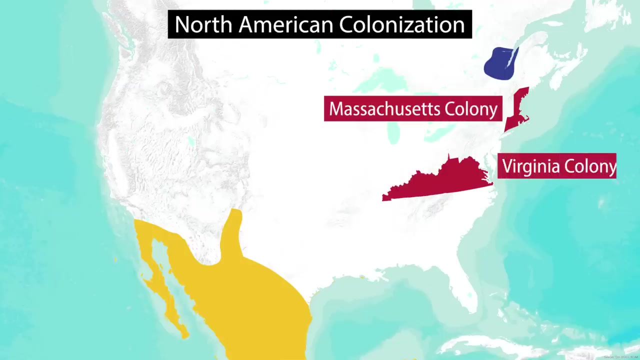 England's first attempt. the colony didn't last By 1590,. the entire settlement was found completely abandoned. To this day nobody truly knows what happened to the nearly 120 colonists. But England persisted and began issuing more charters for more colonies. By the middle of the 1600s, colonies were 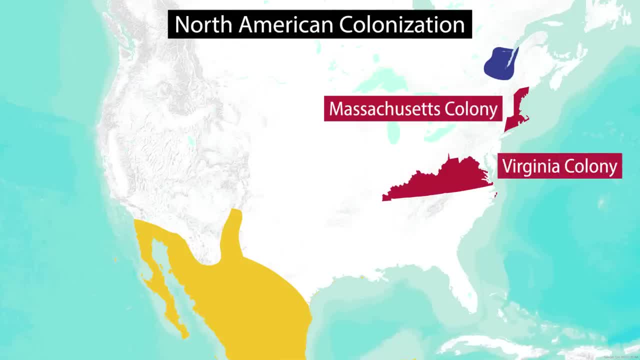 found up and down the east coast of the modern United States. This would include the early province of Carolina, which was founded in 1629. And consisted of the land from the Albemarle Sound in present-day North Carolina to the St 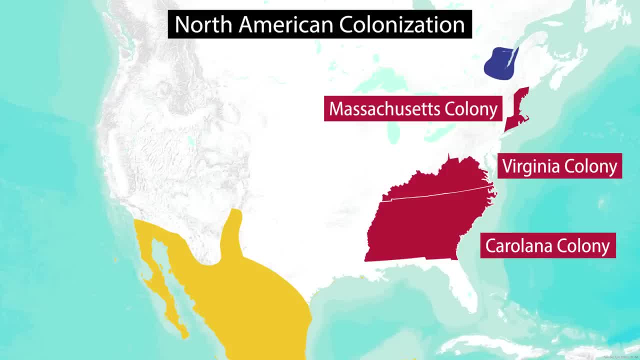 John's River in the south, just below the current Florida-Georgia state line, So quite a bit more than the North Carolina and South Carolina we know today. Unfortunately for Carolina, the colony would ultimately fail. A lack of funding and resources prevented it from growing. and ultimately competing with the colonies of Virginia and Massachusetts, And at the time England found more value in its Caribbean colonies than it did in Carolina. But the colony wouldn't stay gone for too long. Carolina was not a hugely successful start for the area that we would today call North. and South Carolina, But it was an important first step towards the establishment of the two states we know today. But before we get into how two states came from one colony, if you're enjoying this video, hit that subscribe button. More fun geography videos are just a single click away. 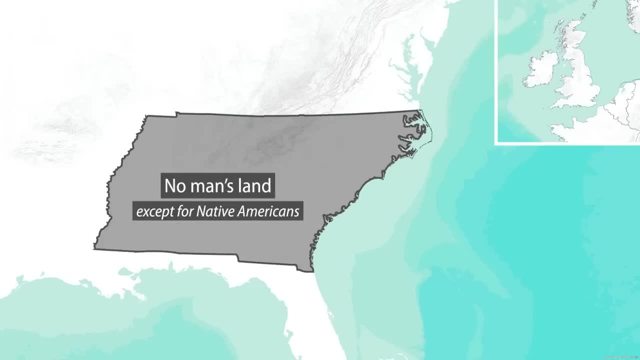 After the colony of Carolina failed, the entire region was left in a state of limbo. King Charles I, who issued the original charter, was executed in 1649. And the original retainer of the charter, Sir Robert Heath, had fled to France. 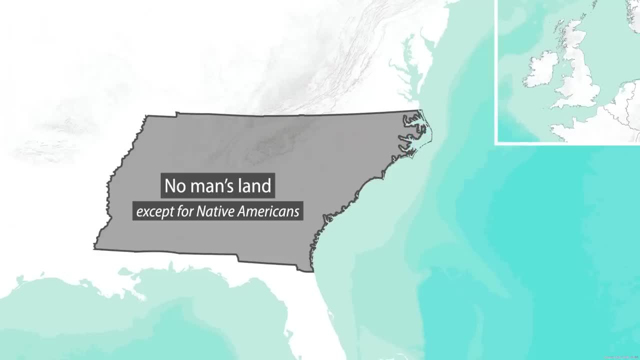 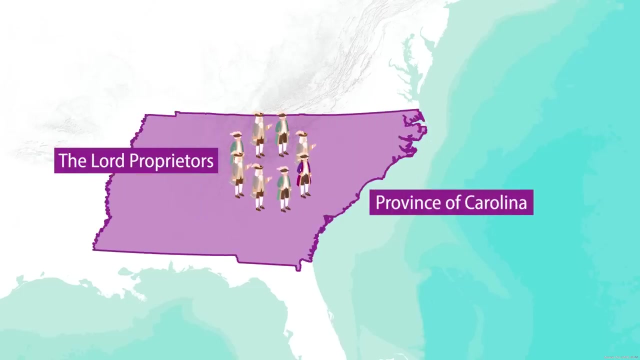 This left the entire region without any sort of owner or occupier. Heath's heirs did try to claim the land for themselves, but the new king, Charles II, ruled the claim invalid. On March 24th 1663, Charles II issued a new charter to a group of eight English noblemen called the Lord Proprietors. 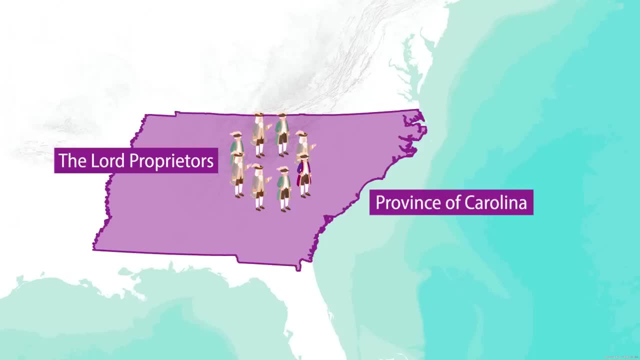 granting them the land formerly known as Carolina as a reward for their faithful support of his efforts to regain the land. Charles II issued a new charter to a group of eight English noblemen called the Lord Proprietors, granting them the land formerly known as Carolina as a reward for their faithful support of his efforts to regain the land. 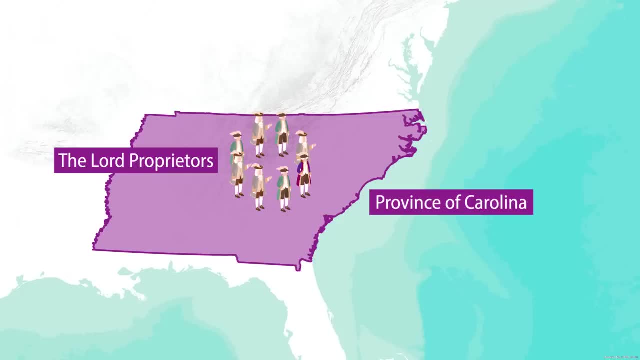 Charles II issued a new charter to a group of eight English noblemen called the Lord Proprietors, granting them the land formerly known as Carolina as a reward for their faithful support of his efforts to regain the land, And during this transition it was renamed to the Province of Carolina. 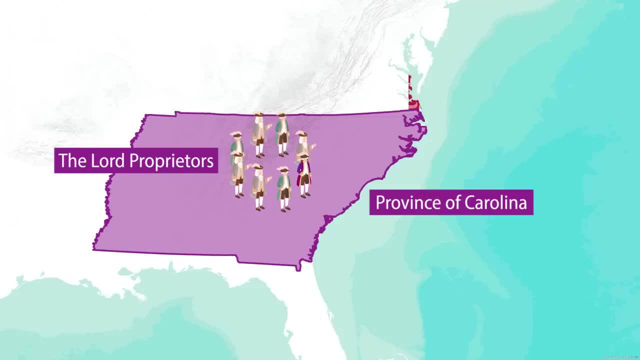 The charter granted the Lord Proprietors title to all of the land from the southern border of the Virginia colony at 36 degrees north to the land at around 31 degrees north. The goal here was to provide a buffer between the successful English colony of Virginia. 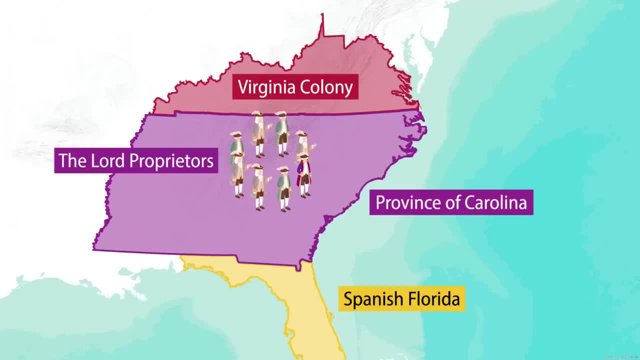 from the Spanish colony in present-day Florida and prevent any northern expansion by the Spaniards. Now, of the eight Lord Proprietors, only one would take much interest in the new province, Lord Shaftesbury, And he had big plans for the new province. 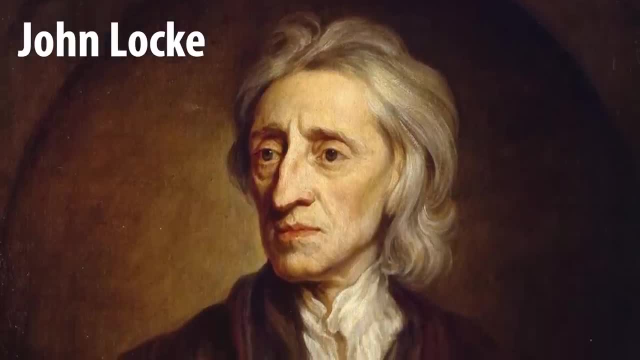 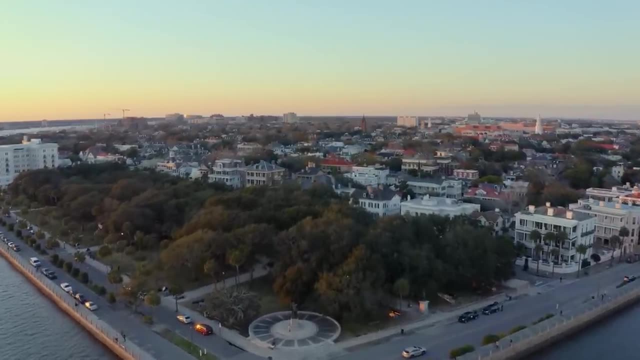 Lord Shaftesbury, along with famed English philosopher John Locke, was set about attempting to create their vision for a utopian society in the Province of Carolina, known as the Grand Model. Really, this was simply a plan for how cities and towns would be laid out. 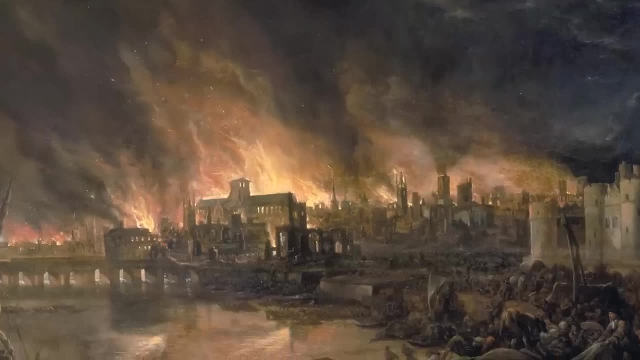 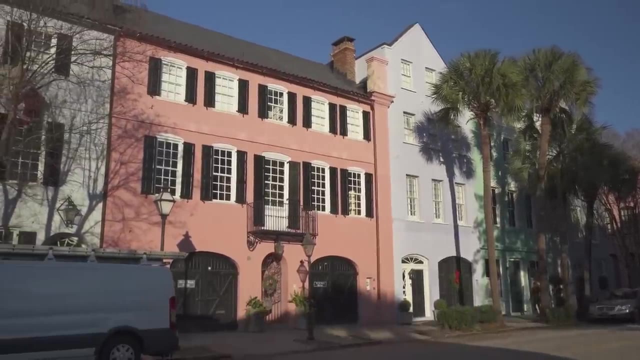 with a particular emphasis to be resistant to fires due to London almost burning down in 1666.. It also factored in things such as public health and safety, land use and urban aesthetics- All things we take for granted now, but in 1666,. 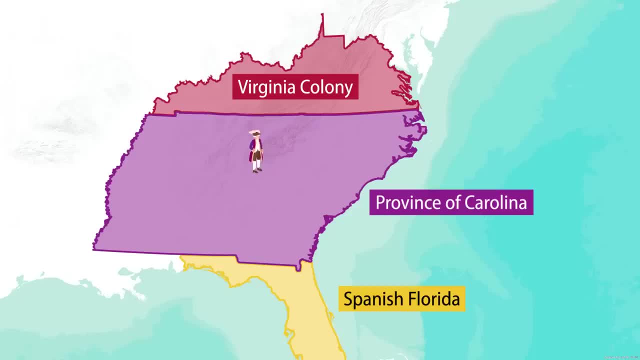 were revolutionary in terms of city and town planning. But while the Lord Proprietors had big goals for Carolina, the reality is that the best laid plans always go awry And in the case of Carolina, it was destined to eventually be split in two. The first thing to know about the split between North Carolina and South Carolina is that there was no single event that caused the divide. Instead, it was really more of a slowly simmering divide that eventually boiled over. That said, we can point to a couple different events. 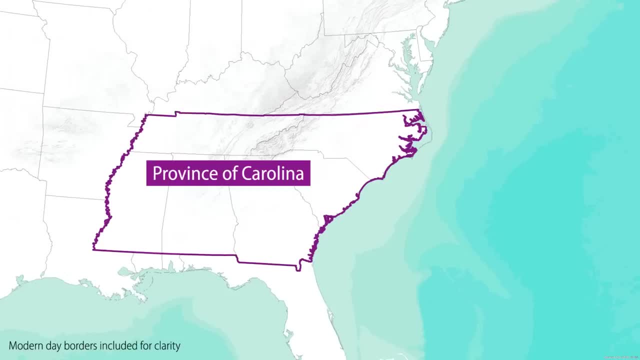 that really spurred the division along. The first is the Tuscarora War in 1711 between the British colonial settlers and the native indigenous peoples of the area. The Tuscarora tribe existed in what is today North Carolina for a long time before European settlers invaded their land And, as one might expect, they didn't take too. 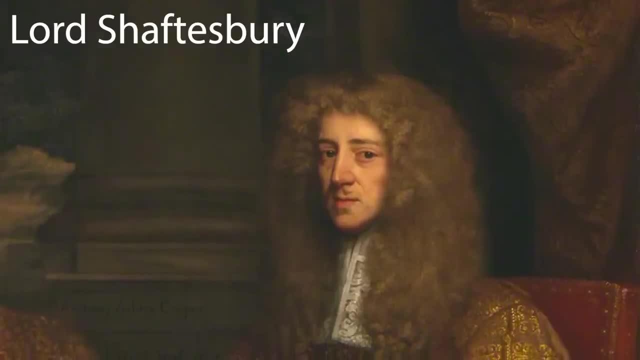 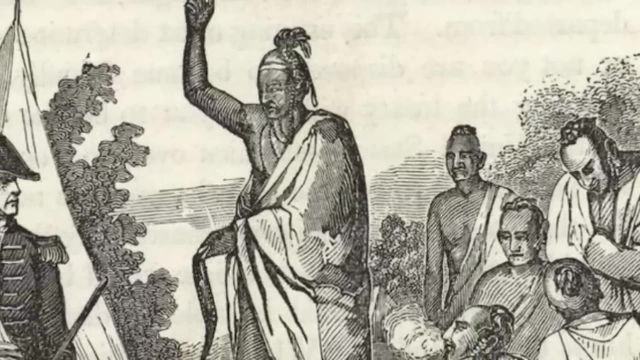 kindly to having their lands stolen from them. More to that point, because the Province of Carolina was ruled by eight separate Lord's Proprietors, the treaties and deals they struck with the tribe were often overruled, ignored or broken by another Lord. 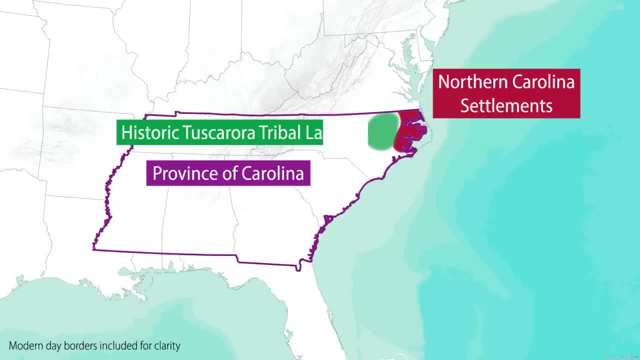 This inevitably would lead to friction and eventually war. The Tuscarora would ultimately lose, but it would build contention in the Carolina colony between those in the North who pulled in more resources to defend the land and those in the South who felt like it really wasn't their problem. You see the Northern part of the Carolina Province and 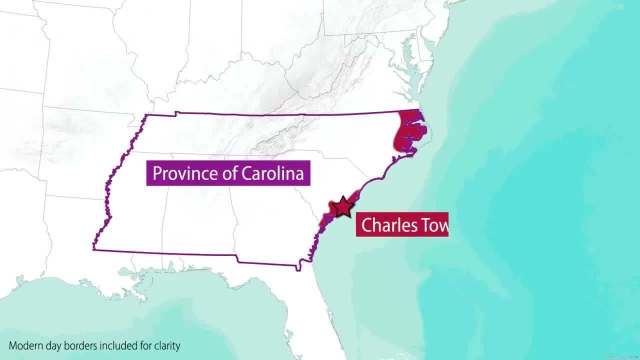 the Southern part were always a bit separate. Charlestown, known today as Charleston, was the capital of the colony, But the Northern area governed themselves independently and had their own major cities in Albemarle and Cape Fear. In fact, both the North and the South had their own governors well before the formal split. 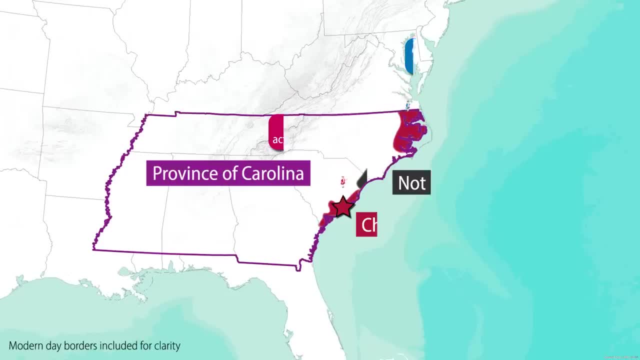 Due to the tensions between the two halves, the Lord's Proprietors' inability to effectively govern the territory and the burgeoning wealth by the Southern part of the colony, the King reclaimed the Southern part of Carolina for the crown in 1719 and left. 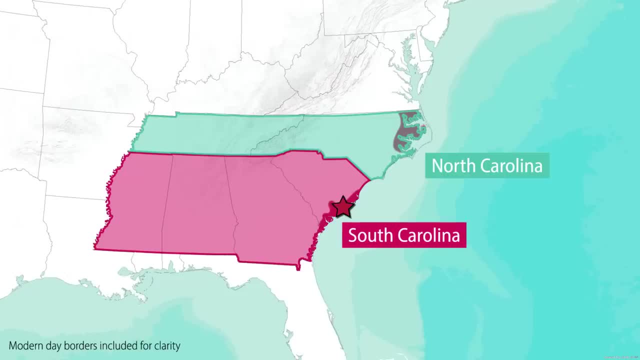 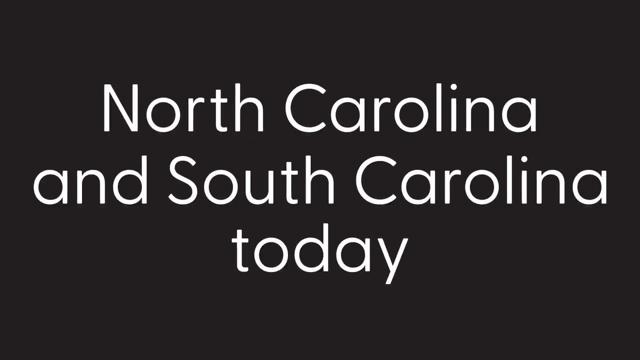 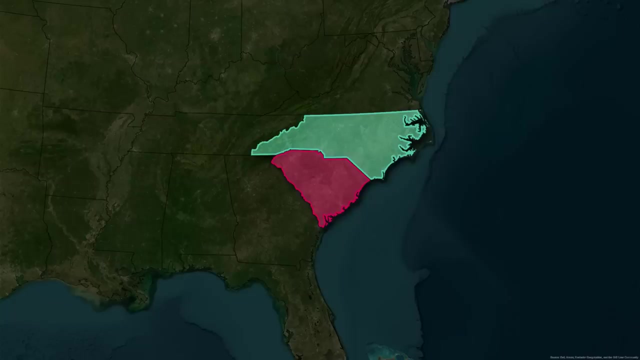 the Northern part for the Lord's Proprietors, And thus North Carolina and South Carolina were officially separated. Today, North Carolina and South Carolina are two completely separate states within the United States, And over the last 300 or so years the two have grown. 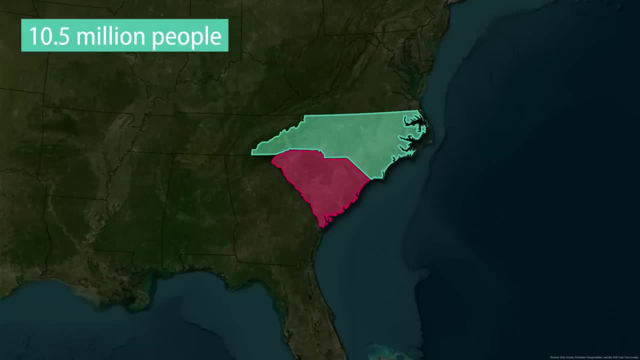 considerably. North Carolina today is home to a little over 10.5 million people, and South Carolina has about 5.2 million people. Of the two states, North Carolina has become the dominant economic engine, with cities such as Charlotte and Raleigh leading in terms of GDP over South Carolina's. 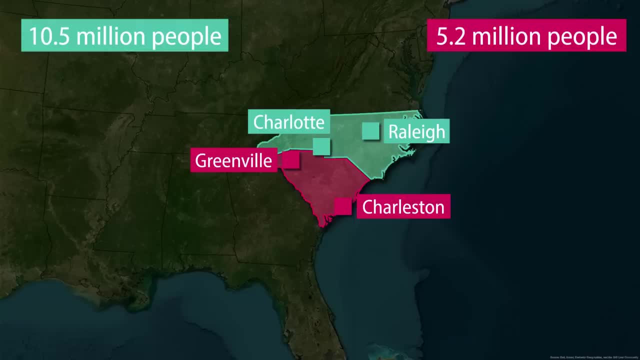 largest city, Charleston, and largest metropolitan area, Greenville, But regardless, the two are very prosperous as of today, with each growing in population by about 10% between 2010 and 2020.. And, of course, because the single province is now two separate US states, it means that each gets